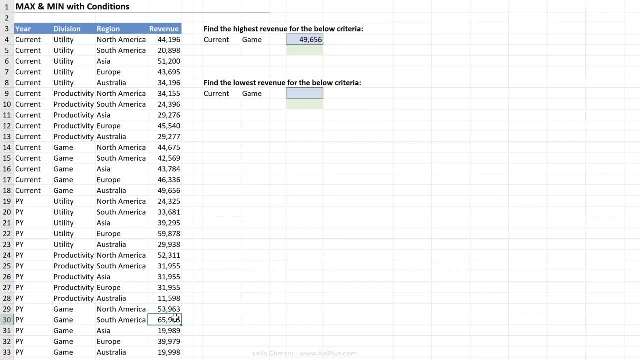 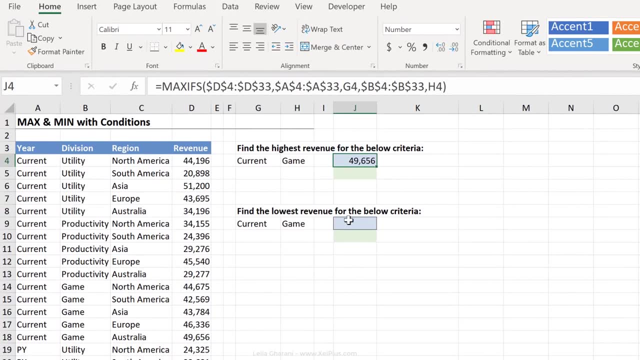 of the entire data set, That would have probably been this: It took a look at these two criteria and gave me the maximum number of these. Let's apply this to get the lowest revenue. So I'm going to copy and paste this here and just change the maxifest to minifest and that's it. 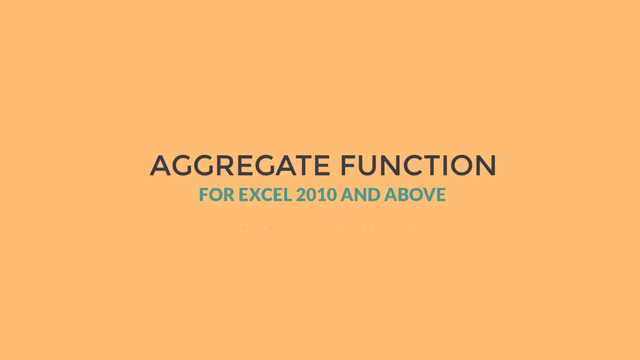 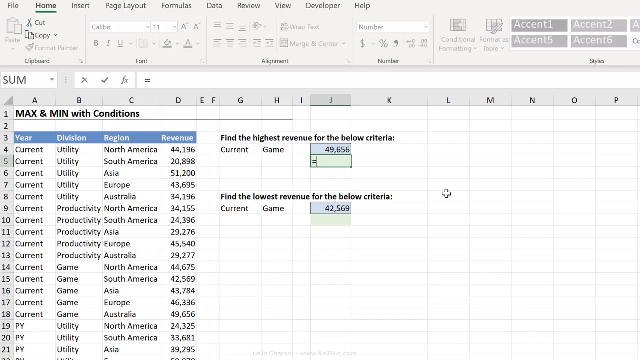 Let's just double check. That's the lowest number here. If you don't have Excel 2016 and above, you can use the aggregate function, which is available since Excel 2010.. What you need to do is start off with aggregate. 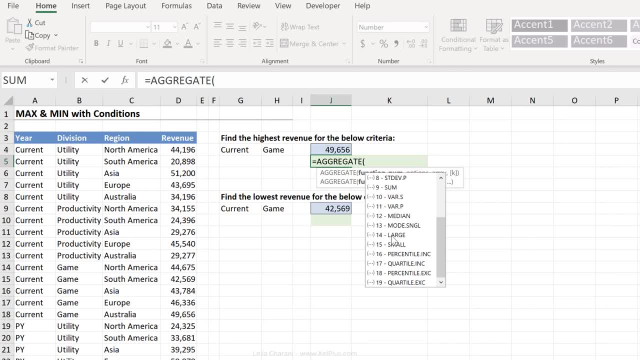 and go with the argument that we need. So for this case, we want to calculate the highest revenue and we go with large. Now, the reason I prefer to use the aggregate function over other functions is because I don't need to press control, shift, enter, because aggregate 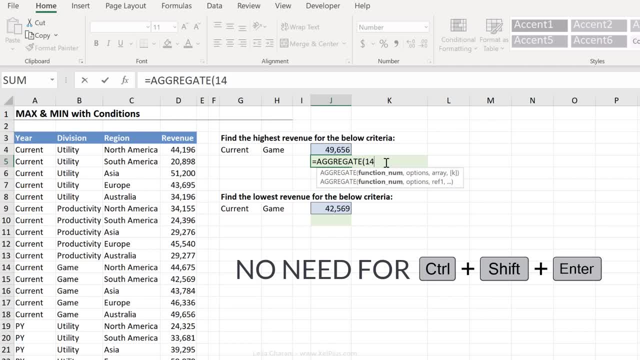 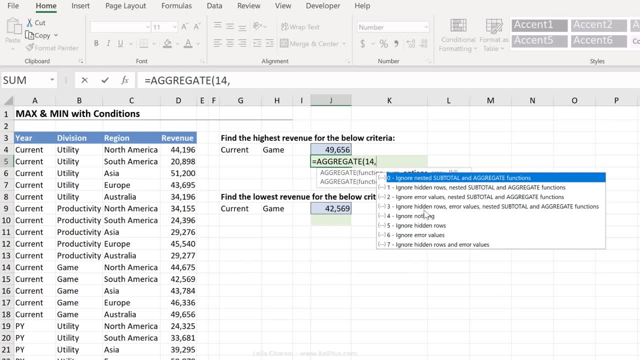 can handle arrays without us having to force it by pressing control, shift, enter. Another advantage of it is the options we get and we get here. You can select whether you want to ignore hidden rows, if you want to ignore nested subtotal. These ones don't matter for us in this case. 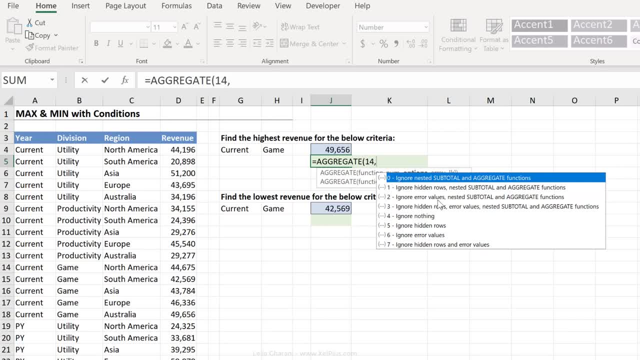 What's going to matter is the fact that we can ignore error values, And you're going to see why in a second. So in the first round I'm just going to select, ignore nothing, and then let's see why we'll need to change it later on. 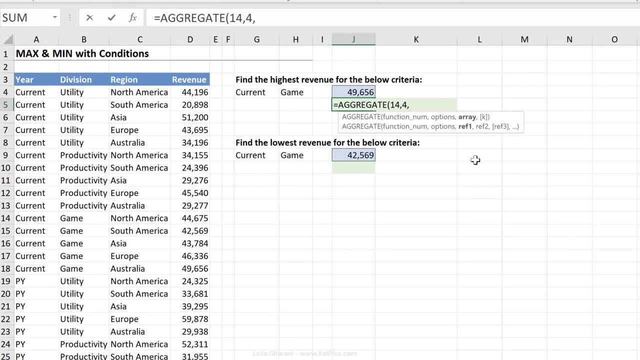 Next argument is the array itself. Here we need to do our logical tests, which means always start with brackets. If you're doing logical tests, you're going to want to make sure that you have all the arguments in your array argument. First logical test is to check if this range here. 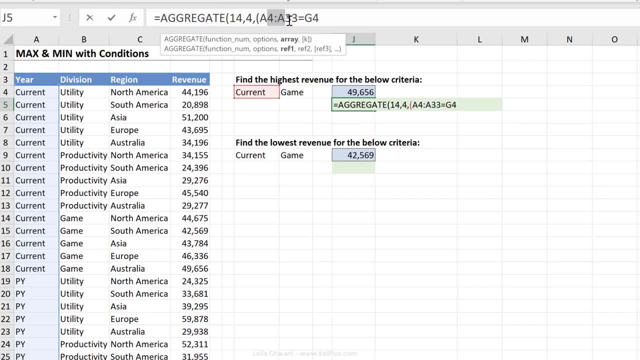 equals this one right here. Now let's do our fixing already here, And I'm just going to close bracket. If this was the only criteria I had, let's just assume I didn't have game, So current is the only thing I had. 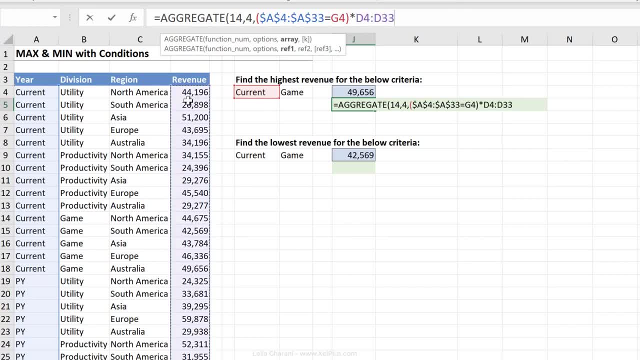 I just have to multiply that result with my revenue range. That's all I'd need to do. I'll show you why in a second. Let me just finish writing the argument. The last argument for aggregate is the K argument. So I have to define if I want the largest. 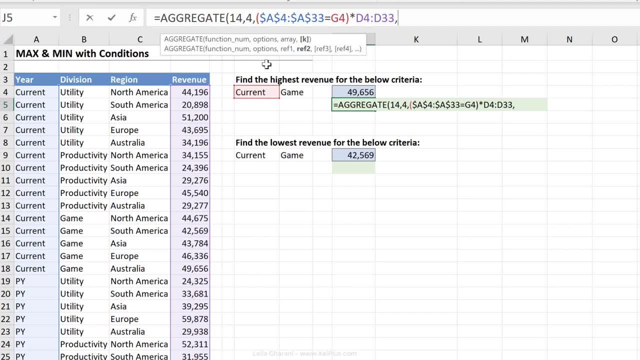 second largest, third largest, and so on. So in this case, what do I want? Always the largest of this criteria right here. So I'm going to close bracket press enter Currently. I've just defined current as my only criteria. 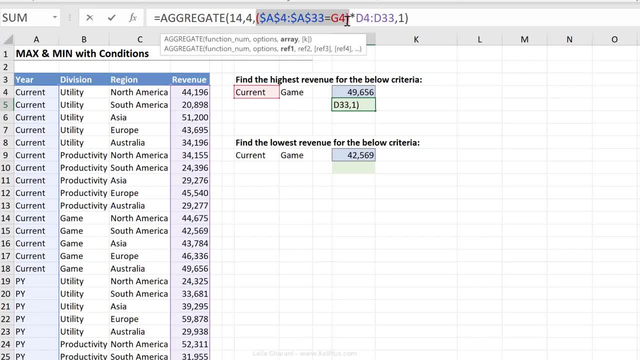 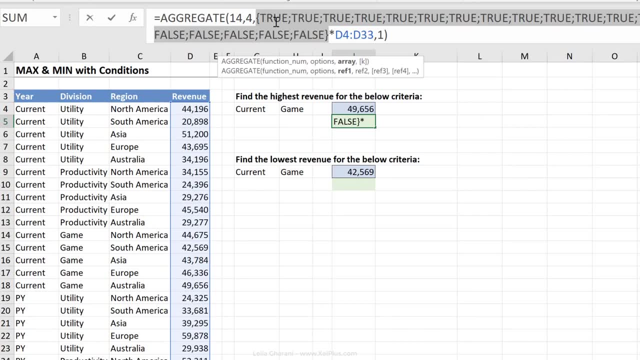 I haven't put in game yet and I'm getting this value. I'm going to highlight this range and press F9.. So F9 key is great for debugging your formula. The result of my logical test is a bunch of true and false values here. 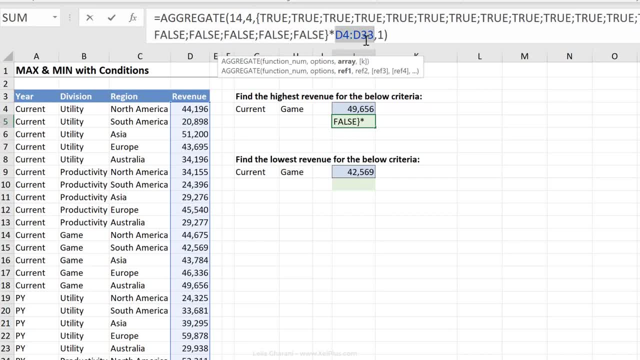 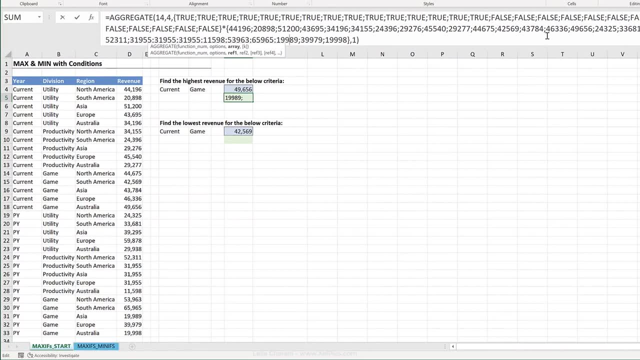 So this means when I multiply the true and false values with this range right here, I get true multiplied with this, true multiplied with this And then, at some point here, false multiplied by the number there. What do I get? Let's just highlight everything and press F9.. 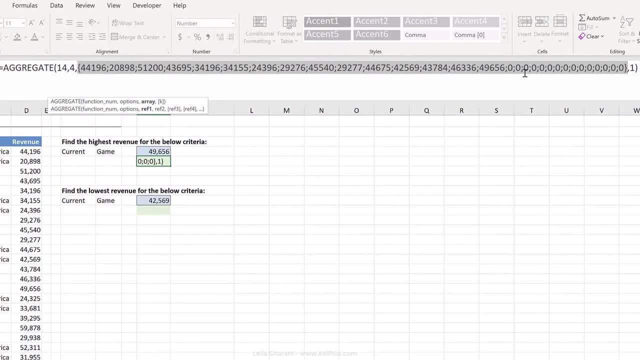 I get my values and a bunch of zeros, because the moment you multiply true with a number, you turn the true into a one, And the moment you multiply false with a number, you turn the false into a zero. So the result is going to be zero. 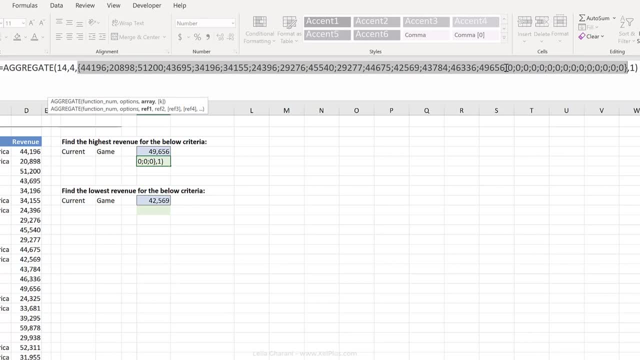 This way, we can see that the result is going to be zero. We can filter out the criteria that doesn't apply by forcing it to become zero, And then we take the max value out of this, which was this number here, And I'm going to press Escape to leave. 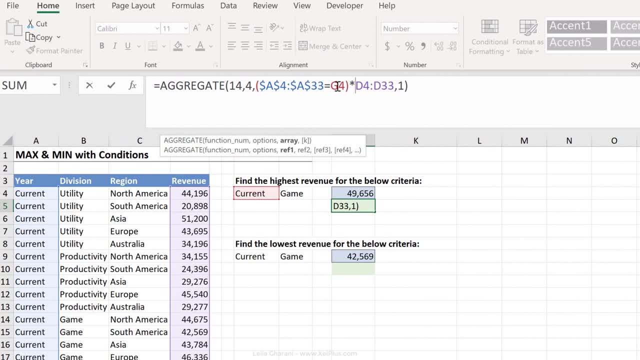 So to bring in my other criteria, all I have to do is multiply this result with the second criteria, So let's just add in the bracket here. My second criteria is to check if division- let's press F4 on this- equals this game here. 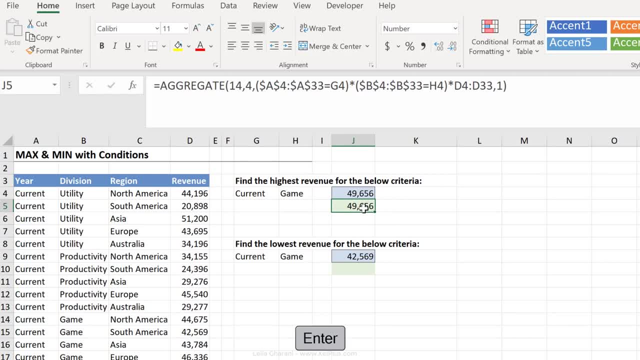 Close bracket and multiply again and press Enter And I get my value right. Because what happens here is this: results in true-false values. This one results in true-false values. Multiply true with a true. What do we get? We get ones. 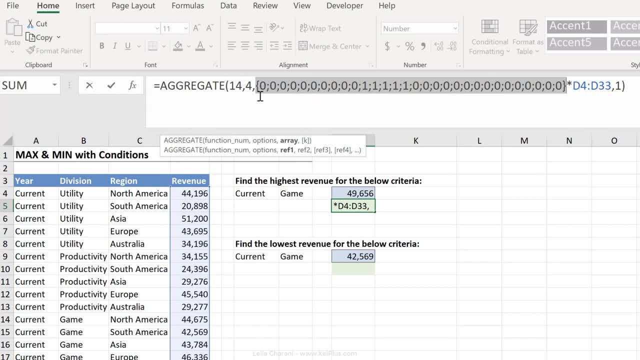 Multiply zero with a true, you get zero, right? So the result of the first one, current utility, is zero, because current was a one. so this was a true. And utility compared to game, it's not the same thing, right. 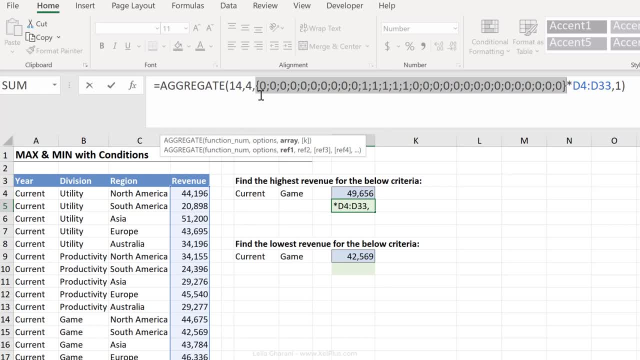 So that was a false. So when we multiplied one with a zero, we got a zero. So I'm going to press Control-Z and go back here. Okay, so let's just fix the last argument here as well, if we're planning to copy it down here. 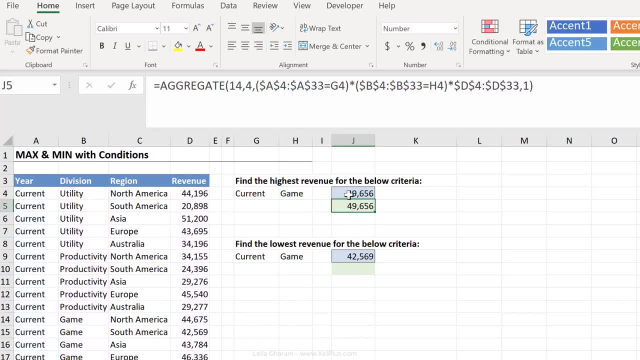 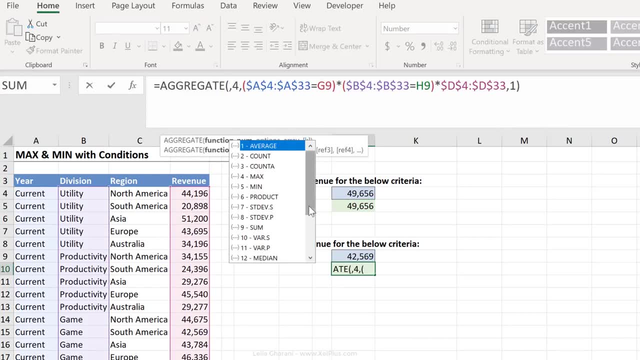 Now, when I press Enter, I get the same value as my maxfs formula. So can I just safely copy this and paste this here and change this to the small argument? Is that going to work? It's not going to work Because, remember, I got a list of numbers and zeros. 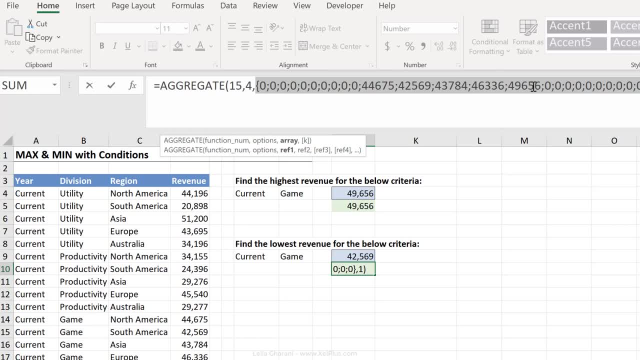 So if I'm taking a look at the minfs- the min value of this- of course it's going to be zero. So I'm going to go back here, Okay. so let's just fix the last argument here as well. 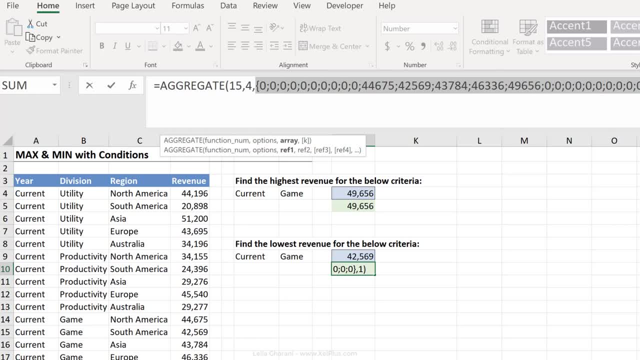 It's going to be zero. So what I need to do is to cancel the zeros out, basically get the minimum value if it's not a zero. And one way I can do this is to force these zeros to become errors, Because, remember, in the second argument for aggregate- 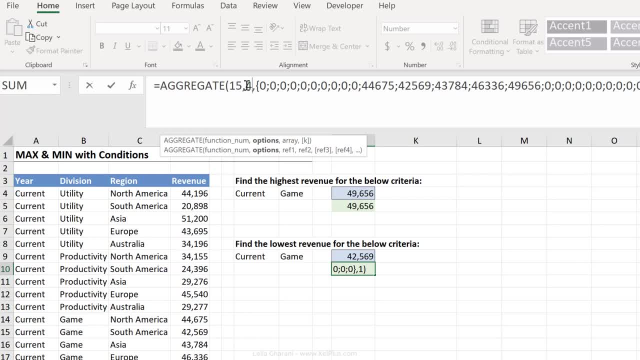 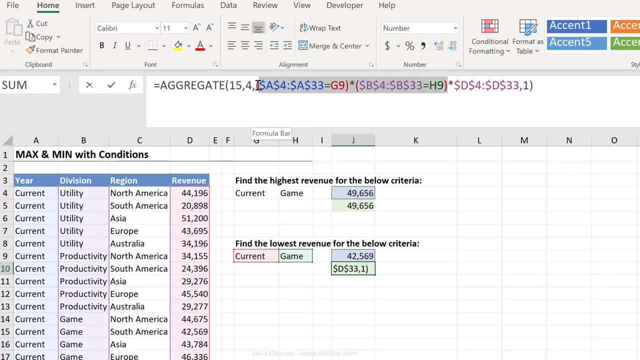 I can say ignore error values. I can't say ignore zero values, but I can say ignore error values. Now how do I force the zeros here to become errors? So instead of getting zeros and ones, I want errors, And once press control Z to go back. 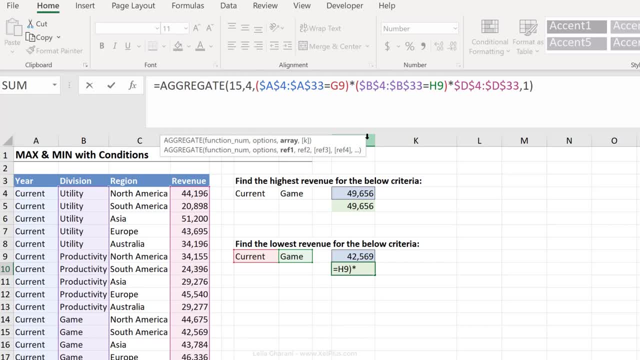 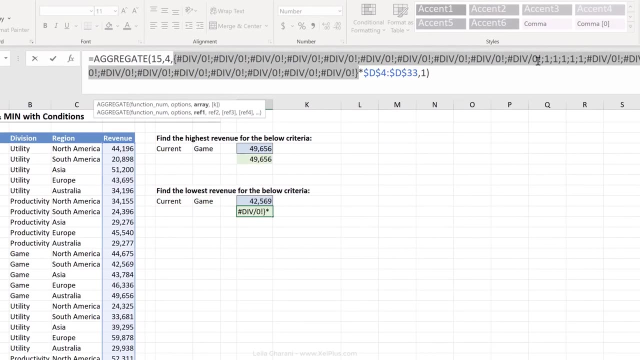 Well, one way I can do this is to divide by zero. So I can say one divided by this part of the array. So I'm basically doing one divided by zero or one divided by one. Now check this out. If I highlight this and press F9, I get errors and ones. 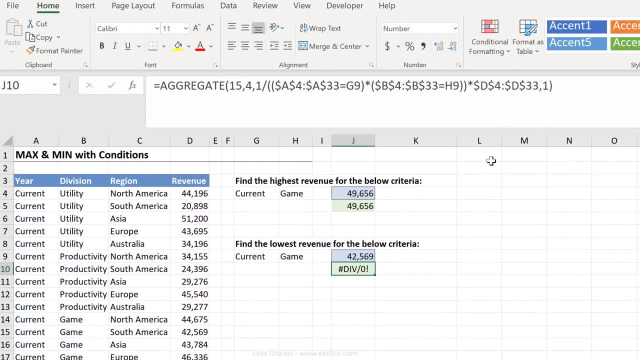 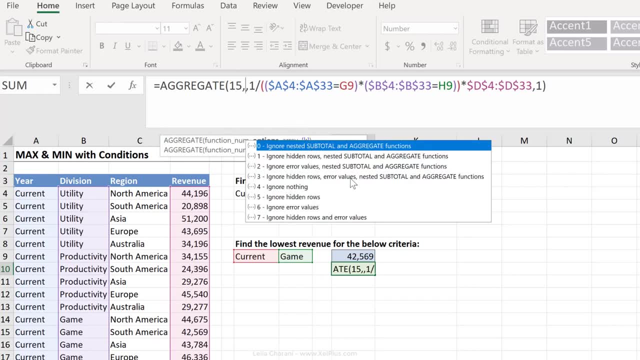 which is exactly what I want. but I'm not done yet, Because- check this out- When I press enter, I get errors. I've told it to ignore nothing. Now I need to update this And say: ignore error values. So any argument that ignores error values is great. 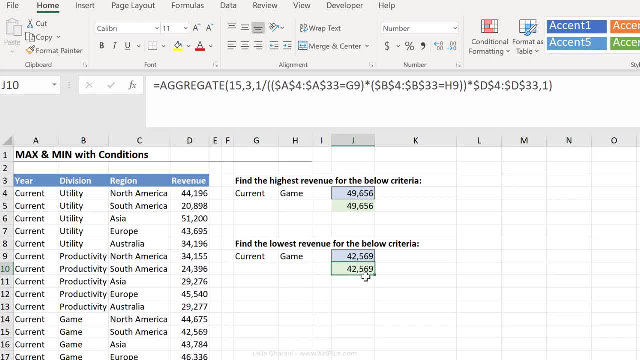 And then press enter and I get the correct results. Okay, so to be consistent, I'm just going to copy and paste this here and just change this to 14.. So those were the two different ways you can use MinFS and MaxFS in your data analysis. 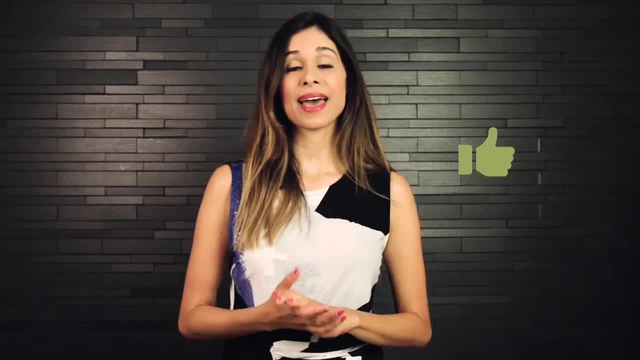 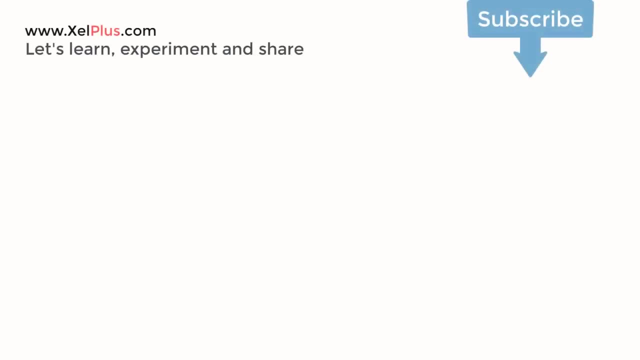 If you like this video, don't forget to give it a thumbs up, And if you want to get updates when I post new videos here, consider subscribing And I'll see you in the next video. Bye, Bye, Bye, Bye. 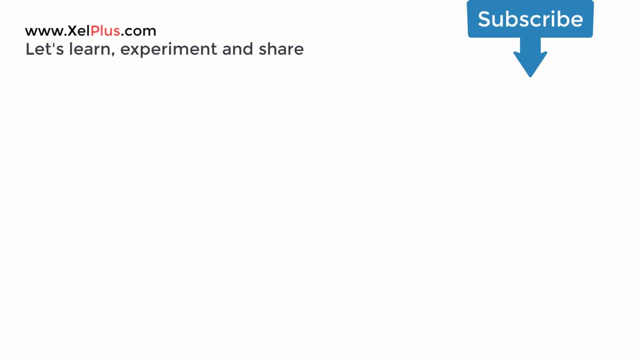